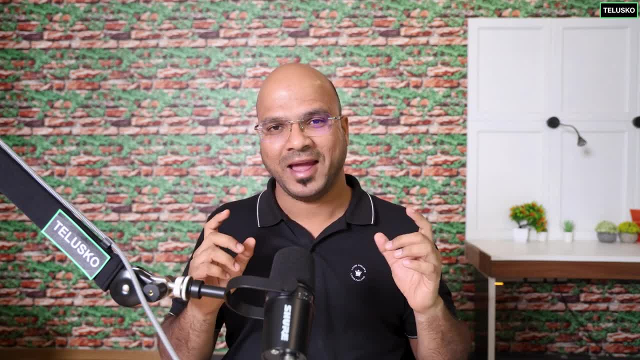 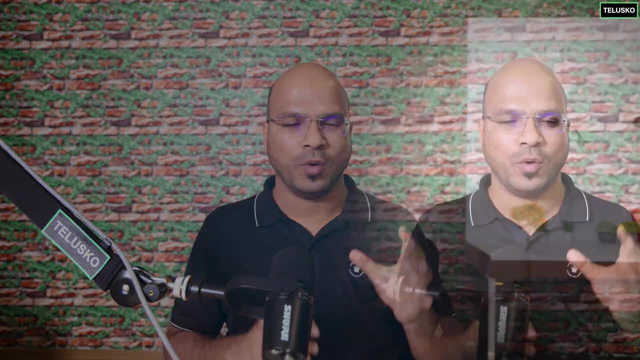 problem. we don't have one solution, we have multiple solutions And we have to pick the best one. Now question arise: how will you choose the best one? So when you say best one, what exactly it means? So let's say, we're on this application. I want my application to use. 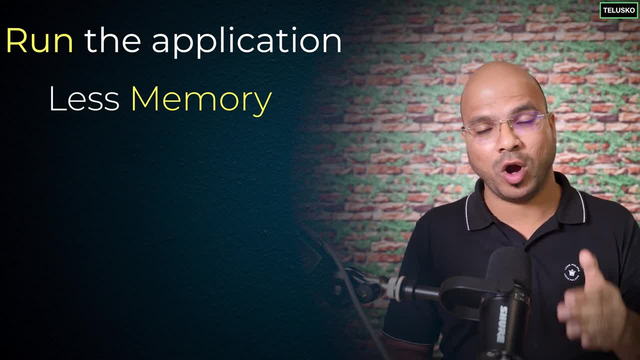 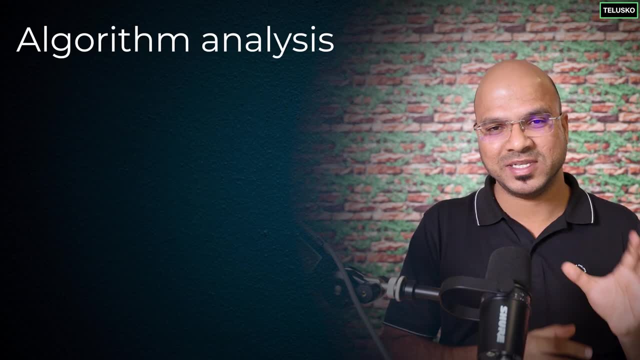 less memory. So let's say, we're on this application. I want my application to use less memory, Or maybe I want, when I run this application, I want it should take less time, or maybe both, And that's why we have this term called algorithm analysis. So basically, 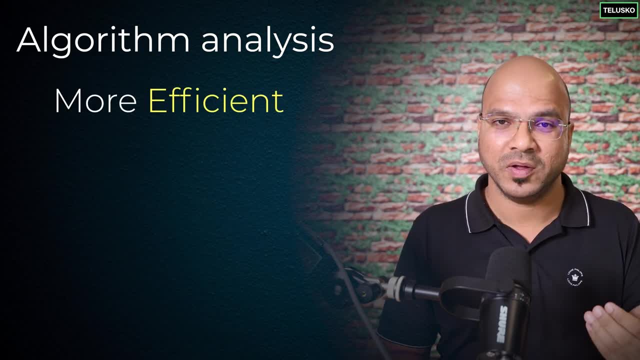 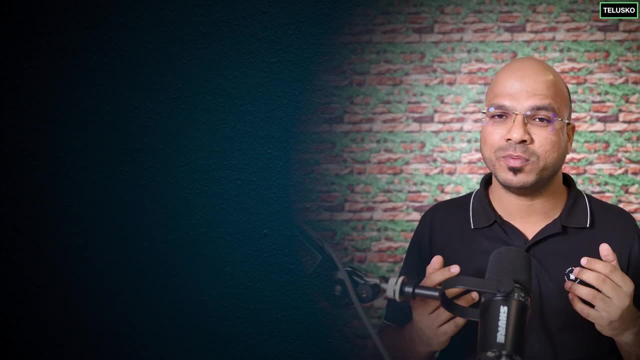 you have to analyze your algorithm so that you can make it more efficient, right, Of course, as a developer, first focus is first the production work and then you think about optimizing it. But when you say optimizing, you have to. you can optimize in two ways. One: 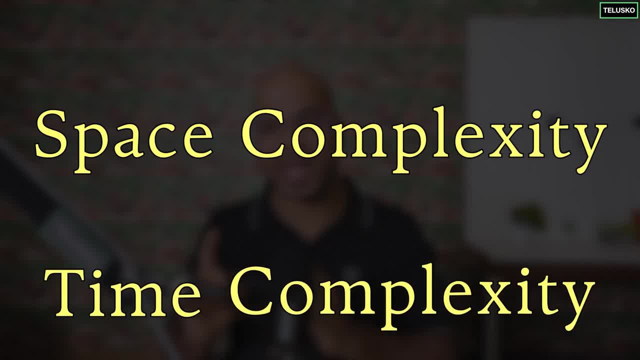 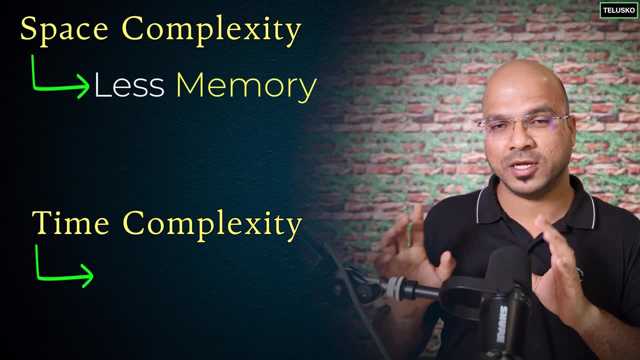 think about the space complexity And second is the time complexity. Space complexity simply means we use an algorithm which will take less memory, And time complexity means it will, it should take less time. But there's one more problem here, And the problem is: how will you calculate the time Or 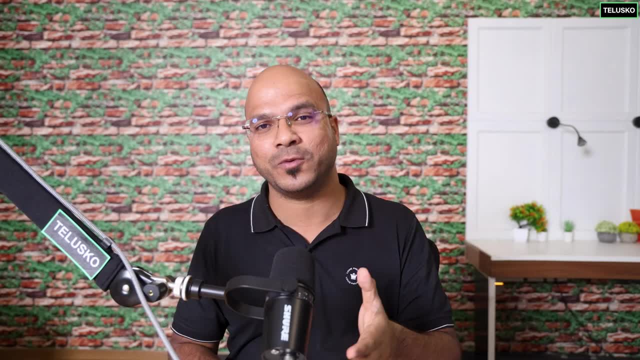 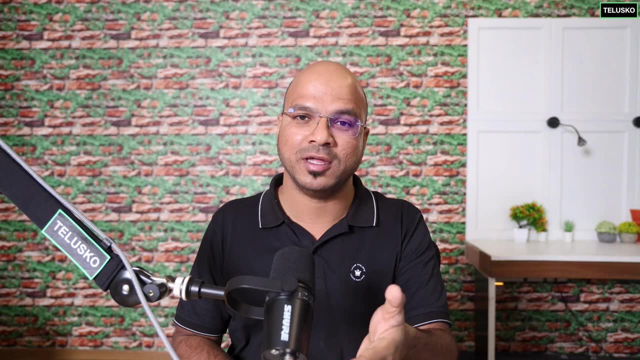 how do you specify the exact time? because every machine will have a different output, right? So if you are testing the algorithm in your machine, it might give you a different time, And then, the moment you test this in your office machine, it will give you a different time. So that's not the. 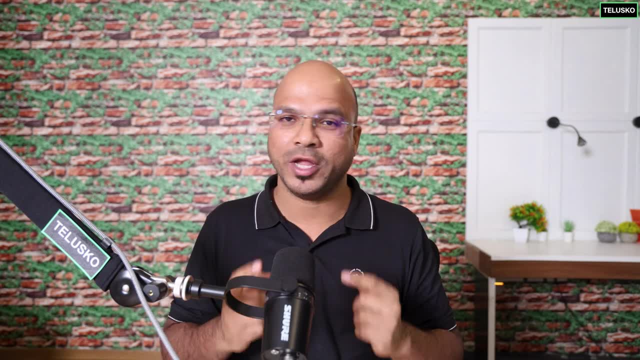 best thing to calculate the number of seconds it takes. But what you can do is there's a way you can calculate with the help of a computer. So let's say you're using a computer and you're going to do a test. So let's say you're using a computer and you're going to do a test. So let's. 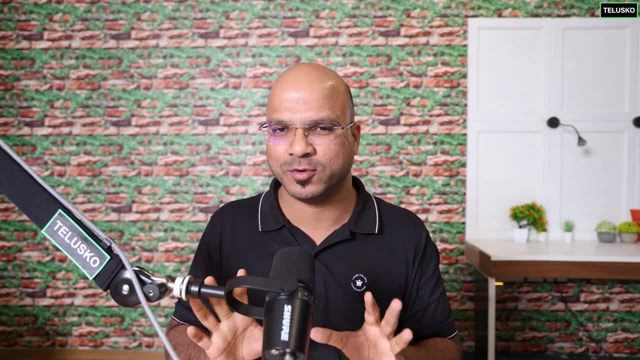 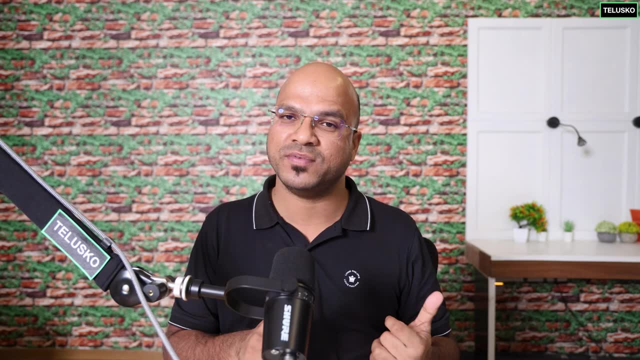 focus on two algorithms here, And then this will make much more sense. So the algorithm which we're talking about now is the searching an element in a sorted array. So in the previous video we have talked about array And then we also talked about the sorted array. So in sorted array. 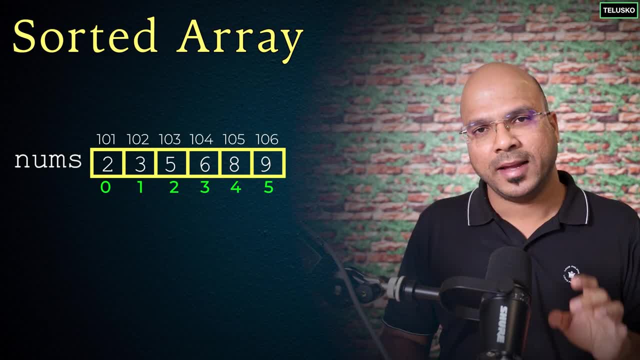 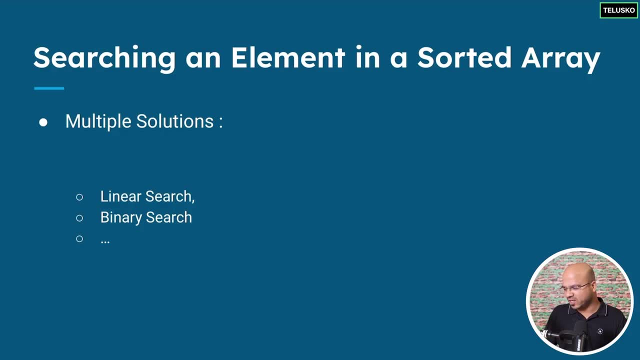 by default. all the elements will be sorted right Now. what I'll do is: I want to search a particular element from this array Now. there are multiple ways of doing it. Let's talk about the two. So, basically, we have an option of linear search, binary search. 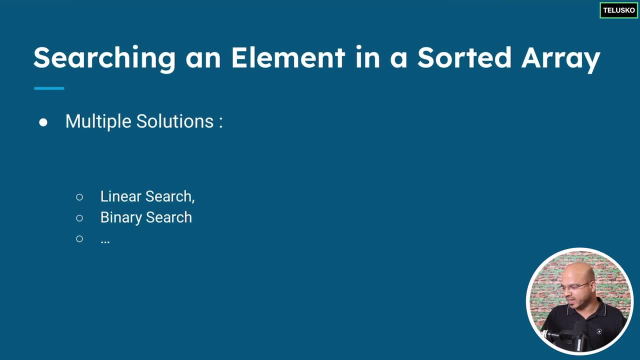 or many more, But let's focus on this too. So what exactly linear search and binary search is? let's talk about that. So what is linear search? So let's say you have an array with you, Okay, so this is your array And in this you have multiple values. So let's say I'm going with 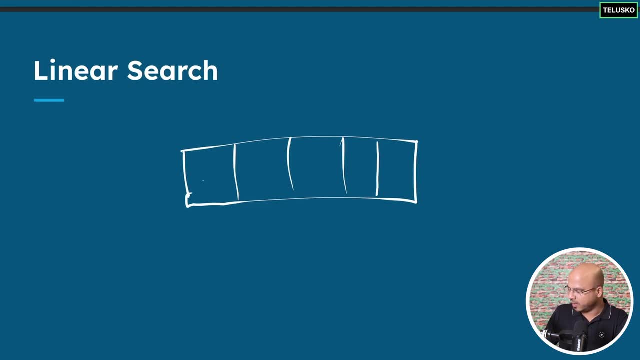 few values here. let's say five values, And then I'm going to write, let's say, 5791217.. So we got this- five values here- right? And then I want to search a particular element. Now this is sorted array, because you can see, all the elements are sorted. We got 5791217.. And I want to search a. 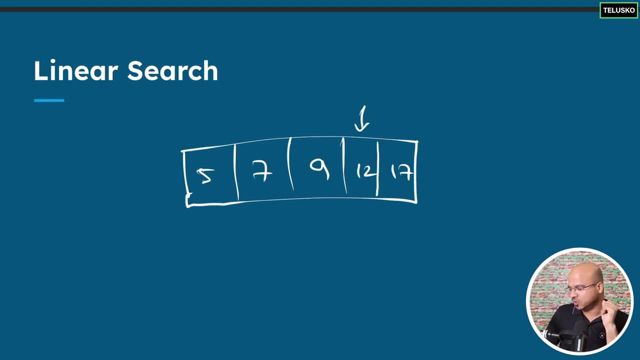 particular element. let's say I want to search 12.. Okay, I want to search this element. So maybe there is a target value which I want to search. In this case the target value is 12.. So I want to search 12, right, And then this is an array. So what we do in the linear search is: you go one. 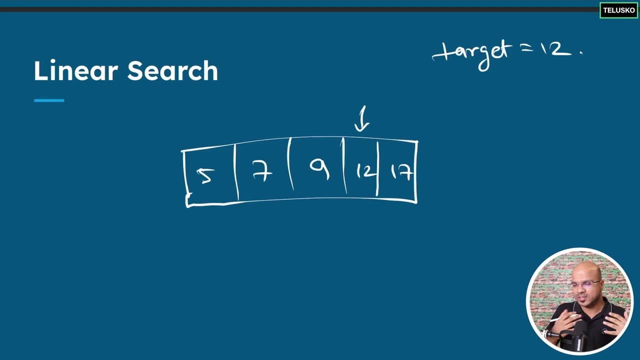 by one. So what you do is in fact, we have talked about this in the previous video as well, So we'll make it a bit faster- So what you do is: whatever your target value is, you will compare that with the first element. If it is matching, then you will compare that with the first element. So if it is, 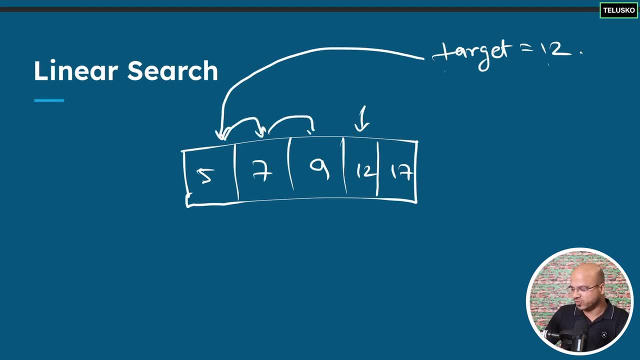 matching, then you will compare that with the first element. If it is matching, then you will compare that with the first element. So if it is matching, then you will compare that with the first element. Great, Otherwise you will move to the next element. Otherwise you will move to the next. 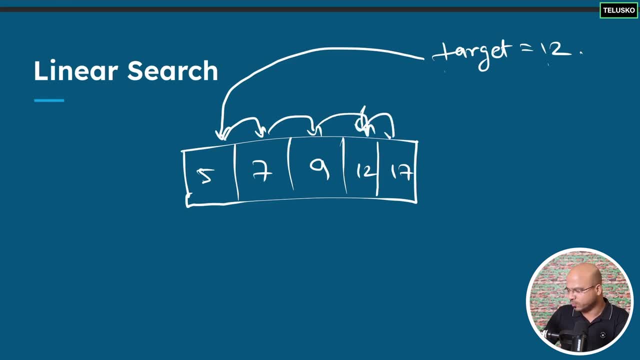 element, Otherwise you will move to the next element, And I mean, of course, at this point we don't have to go to the next element. So here we basically got the value, And once you got the value, you can return the value. right Now there's a problem here. The problem is what if 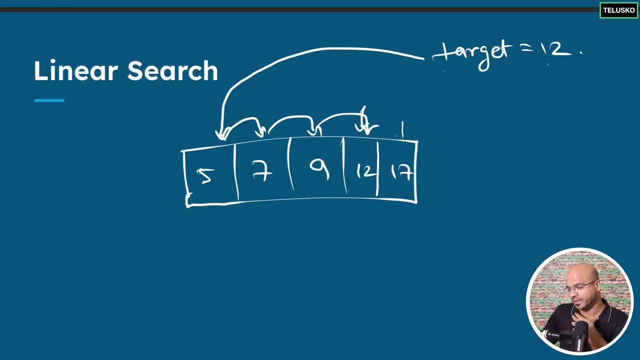 the element is not there in the array. So of course you have to reach till the end. Okay, what could be the best way scenario here? So let's say you're searching for an element. let's say element is five, And now we know element five with the start itself. So when you have the 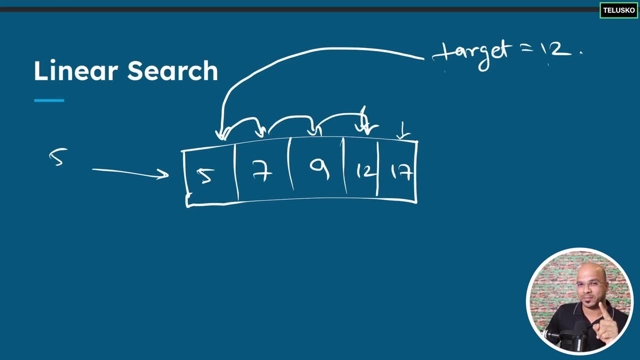 element at the start, it will take only one step. But what if you have element at the end? so it will take. the steps depend upon the length of the array. So let's say, if you have five values, it will take five steps. When you have 10 values, it will take 10 steps. When you have 1 million. 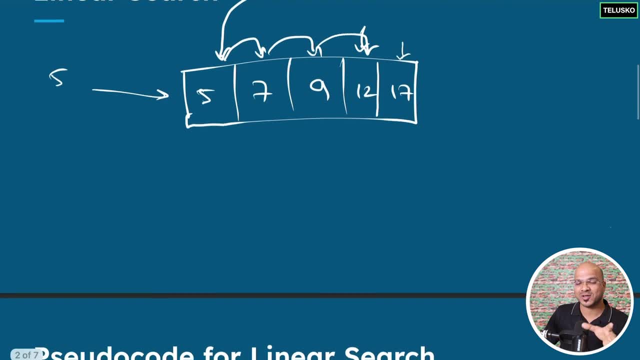 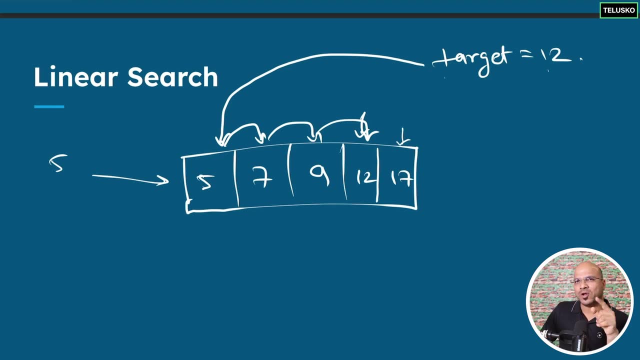 values. okay, that's huge. Let's talk about 1000.. So let's say, when you have 1000 values, it will take 1000 steps. That's tricky right Now. the problem is not, it is taking 1000 steps. 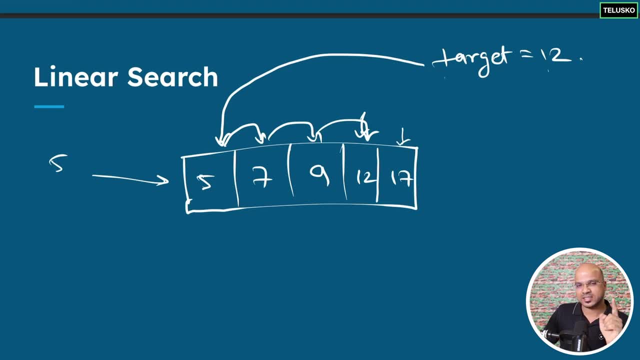 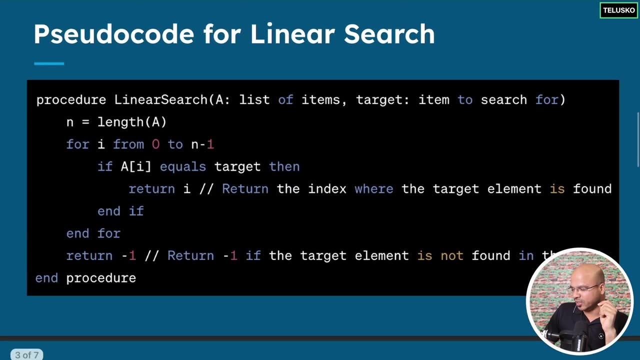 The problem is, as your size increases, it is also increasing the number of steps to search. Okay, that's one parameter you have to remember. So that's a theory. right Now, let's understand that with the help of a pseudocode here, So you can see I'm writing a pseudocode. Why pseudocode? Why not some? 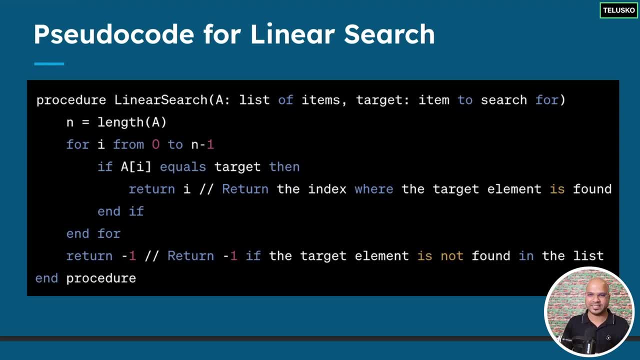 programming language. syntax here is because we wanted to make a generic so that you can doesn't matter in which language you work- maybe C, C++, Java, JavaScript, Python, maybe COBOL. your choice that this could pseudocode remains the same right Now. 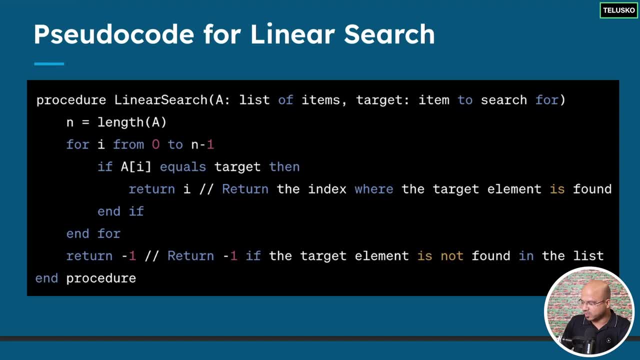 this can be function, procedure doesn't matter. So what I'm doing is doing doing here is: we have a procedure, right, it can be a function, And the name of the function here is the linear search. Okay, Now we are accepting a list of items. Now, this is your array. 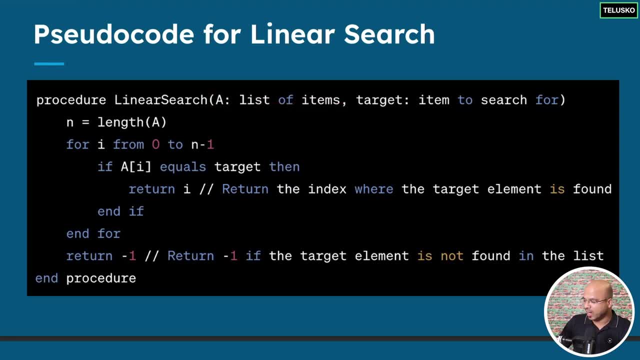 the name of the array is a okay. And then you are also passing a target, what you're searching. So in this case we were searching for 12. But doesn't matter. So you have an array with multiple values. it can be one value, 10 values, 1000 values, doesn't matter. And then you're also 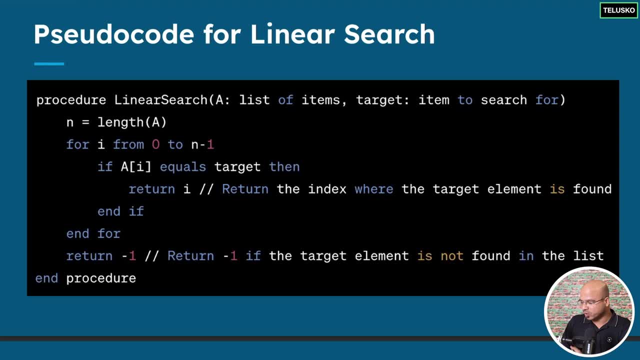 passing a target. what you want to search? Now you will go inside this And then for the first thing you will do is you will want to find the length of the array, because of course you should know right till when you have to search. So you've got a length which is stored. 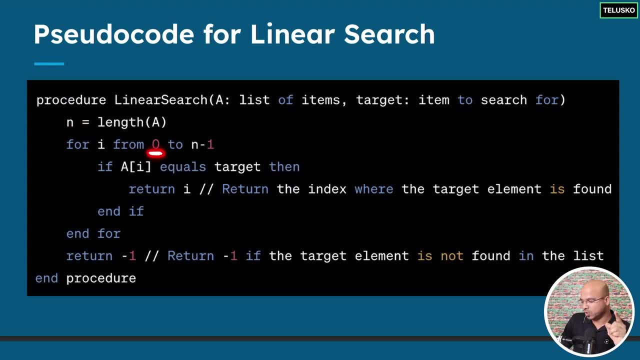 in the end. And then we are going to basically going from zero to n minus one, because we, when you start with zero, you have to end with one less right. So if you have 10 values, you will go to zero, to nine. So you will go from the first value to the last value And then you will search. 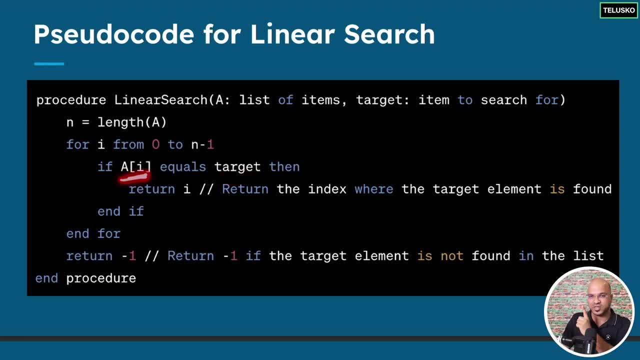 for the next value, And then you will go to the next value, And then you will go to the next value. So when you're searching for the first element, that's the first element. here, target is matching. if, yes, you're good, you can simply return the value. But what if you're not? 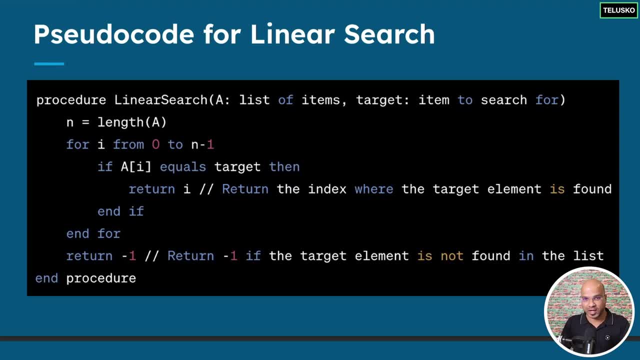 magic is not matching, it will go for the next iteration. next value: Is it matching? Yes, good return. What if it's not matching? next value? So basically you have to search each value till you're not finding it. So that's basically a pseudocode here. And what if there is no element? 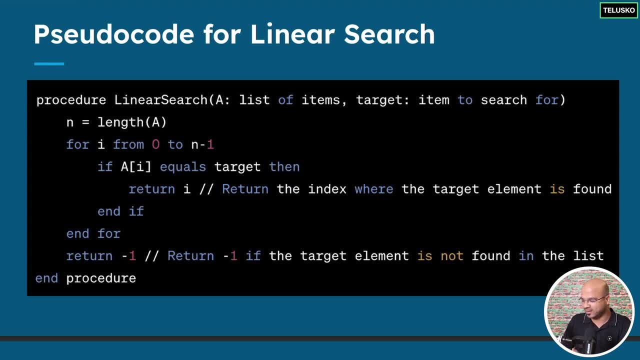 example, you have an, you have five values and you're searching for a value which is not there. you can return minus one by specifying: hey, the value is not there. This is simple linear search. the code is small, but then the time complexity, which is the number amount of time it takes, is. 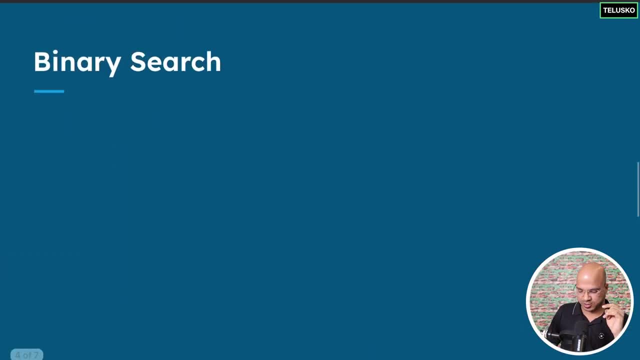 huge. Okay, now let's go for the second approach, which is your binary search. Now, what happens in binary searches? it's very simple. Basically it's not that simple, But let's say so. what you do is you have an array, again a sorted array, And let's say we have multiple values here. I'm not sure how. 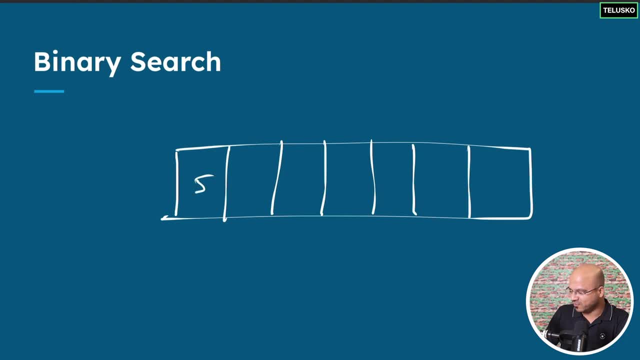 many lines I'm going to draw, So let's count it later. So let's say we got five year, again six, eight, nine, 1113, 17.. Okay, so I maybe. I love odd numbers, So it doesn't matter what values you have. 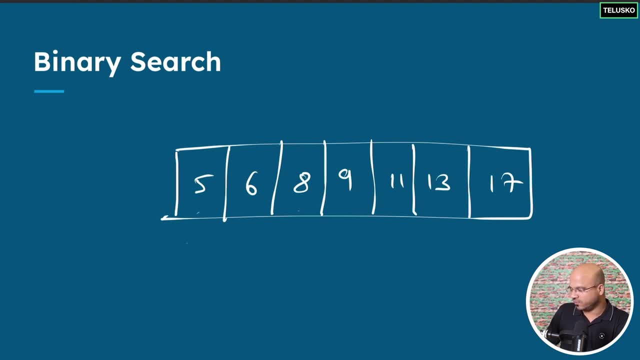 there. So we got 1234567.. So we got seven values. right Now what you do is in binary search. Now, since this is sorted, if you're searching for a particular element, let's say I'm searching for eight here, okay, and we know eight is here. we know it, but computer has no idea where it is. 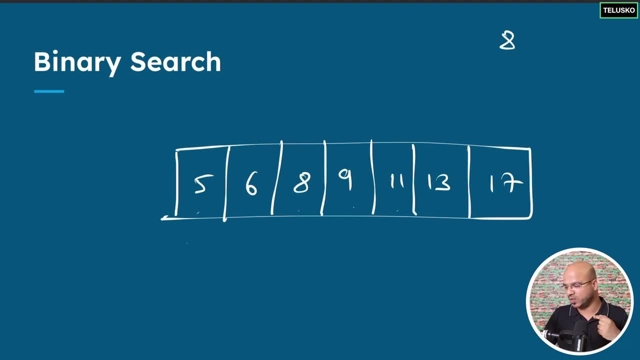 So how it is going to search Now in linear search what we were doing is we were jumping, basically, from value to value, searching, checking this, checking this and then look, goes on. So now I just call it one is because you divide your array into two parts, That's the binary is now. 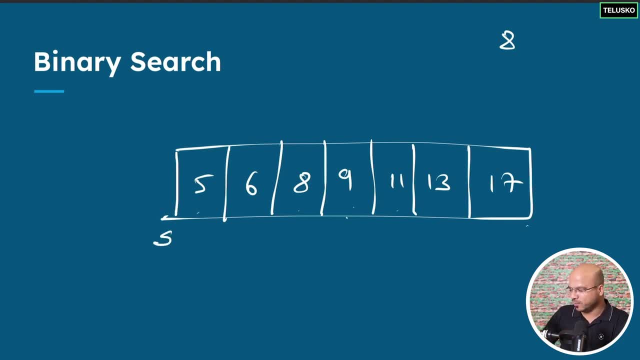 how you do it. So basically what you do is you give a starting point and then you give a ending point And of course every element here will have an index value. So in total here we got a seven values right, which goes from zero to six. Now what you do is you first divide your 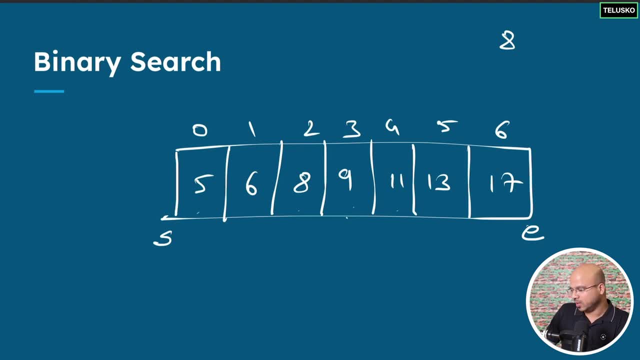 array into two parts, And to do that we have to find a mid value. Okay, so, even before you divide, you find a mid value. So how do you find a mid value? So mid value is equal to the starting position plus ending position divided by two. Okay, now this is six divided by two, which is: 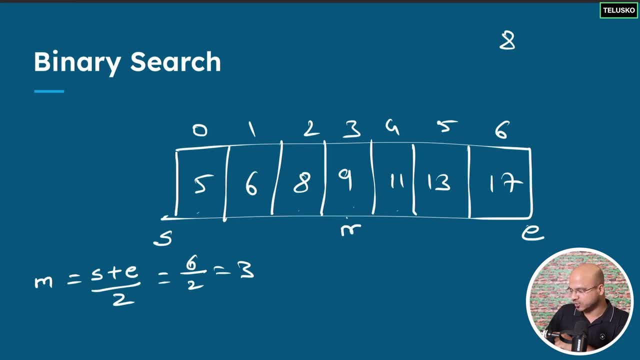 three. Okay, so your mid now is three And this is your middle. Okay, Now, basically, you check with the middle. Okay, you always check with the middle. is the value which you're searching for, which is here? is it matching with the mid value, which is nine? No, it's not matching, But is it less than or? 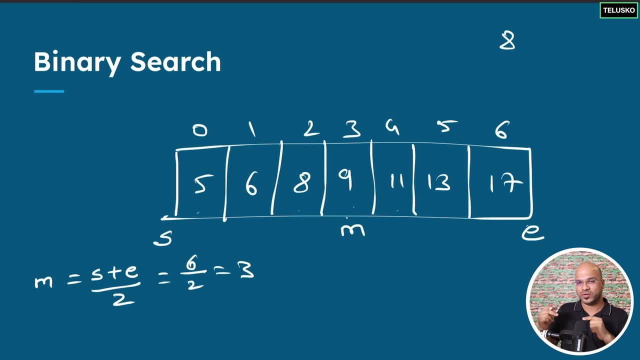 greater than. if the value which you're searching for is less than the value which you got as a mid value, then the values after the mid value is of no importance, right? So this values here has no importance. you can directly skip them. So you can divide your array into two parts. 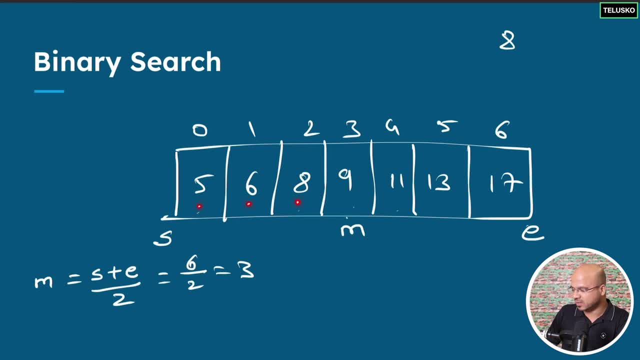 So you've got the first section here, which is five, six, eight, nine, And then you've got the second section here, which is 1113, 17.. So what you can do is you can basically skip this part, or maybe we'll just do that with a color. Now we can skip. 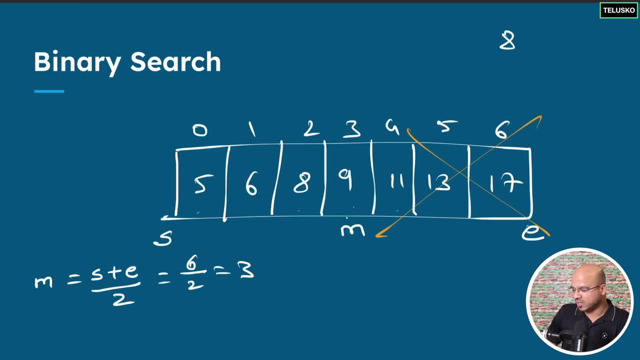 this part. we don't need this value. the value which you want to focus on is 5689.. So what you do now is you make your mid as the end okay, because we have shifted to the left part of the array Now. when you after, of course, when you shift to the right part of the array, in case 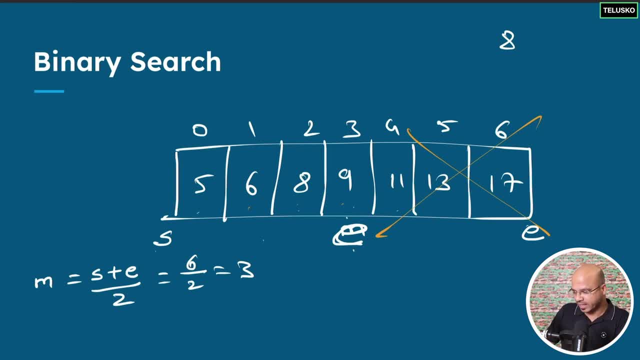 then you shift your starting value. Now here you can see that you can shift your starting value. Now, here you got s and e again, And then what you do is you again check your ending. you will find your new, new mid value. So again, s plus a divided by two, now s is 00 plus three is three by two. 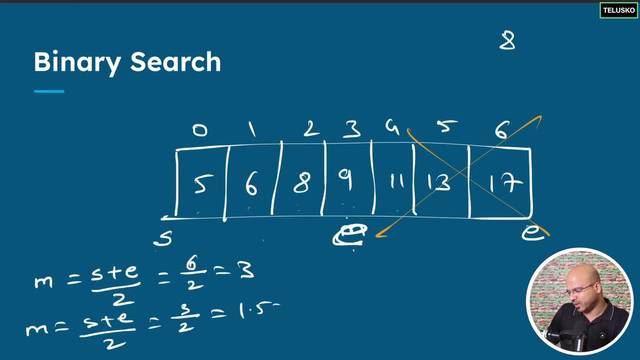 which is one. Of course you can say 1.5.. But let's say this is one equal to one. we can apply a float function to get the nearest integer. Okay, so we got one here right. So what you do is you. 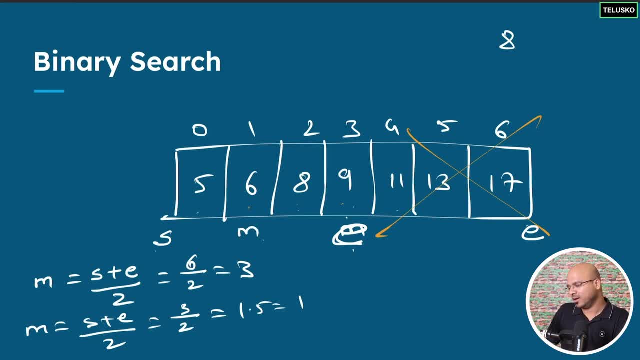 check. So this is your mid. again you check: is it matching with the value? No, it's not matching, So it is not matching with six. then what you do? then you again divide your array into two parts, but then which? which one you have to skip now? Now, now we know that the mid is six, So we have. 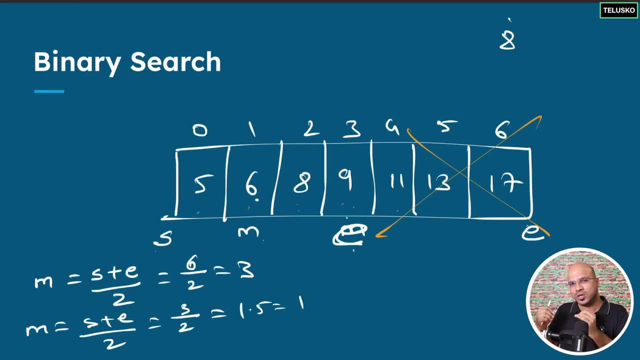 to jump to the next value. I mean we have to look at the right side value. So six is less than eight, right? So I have to look at the right side. So now what we're going to do is: let's we have divided. 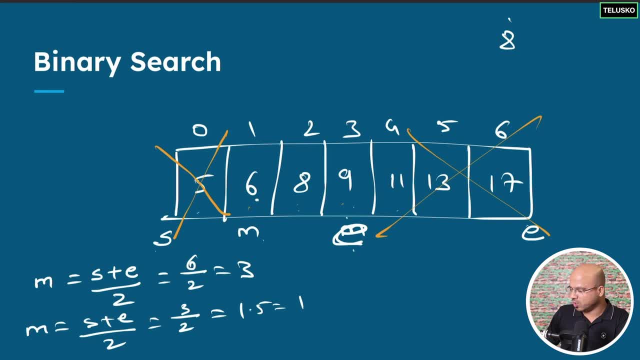 into two parts, right. So now we can skip this part and focus on the right side now. So your starting position has been moved here now. Now this is your s and you got e. So again you will find a new mid, which is s plus e, divided by two, which is a one. 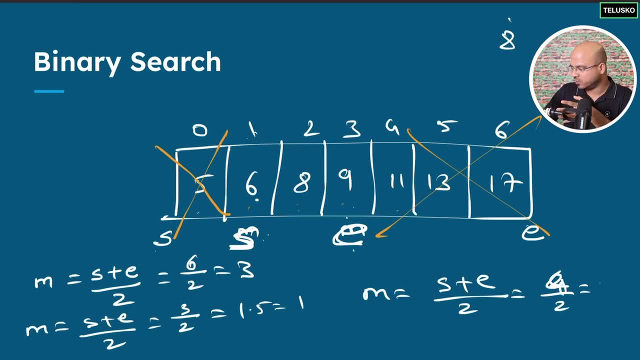 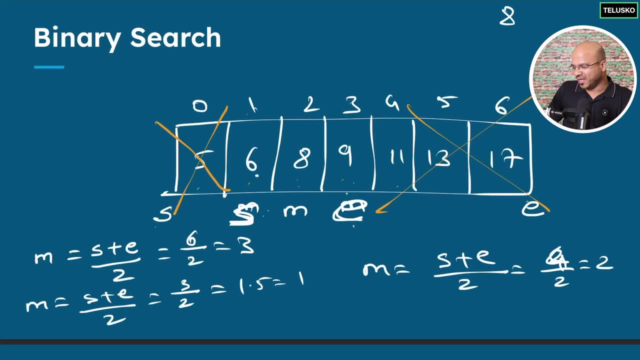 plus three is four. four divided by two is equal to two, So your mid now is eight. Now is it matching? Yes, Okay, And that's how you got the value. Now, if you might be thinking we have done so many, 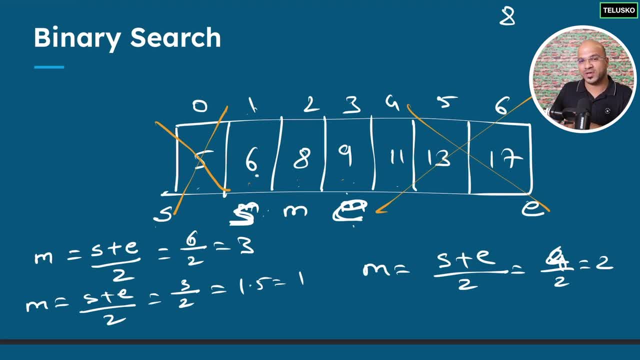 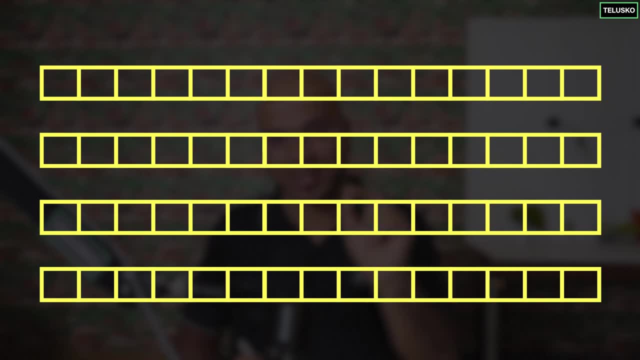 steps right, Not exactly Basically, at the start itself, we have removed half of the array and which is very important, right? So let's say, if you have an array size of 1000, at the start of the first operation you have removed 500 values For the next operation, when you do. 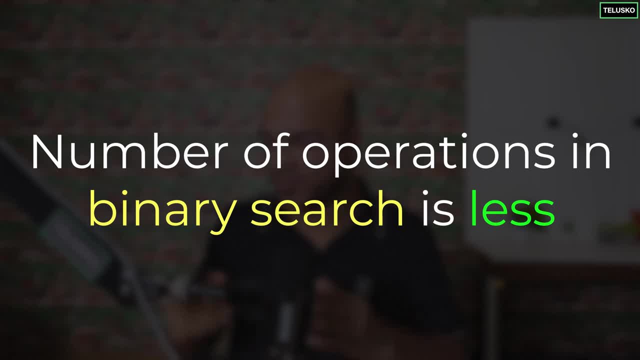 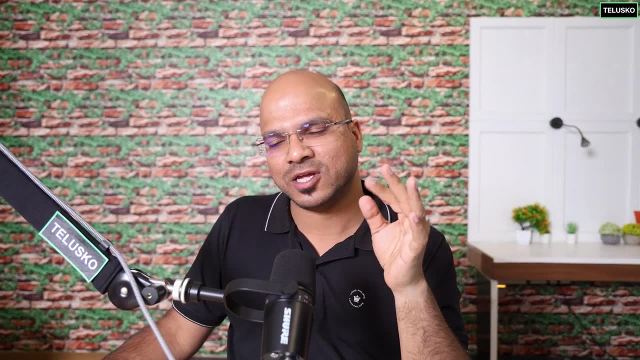 it you remove 250 values, So the number of operations which are doing with binary search is less right, And that's how you know that this is better than the linear search. Of course, in linear search, if the value which you're searching for is the first value, it's very fast. 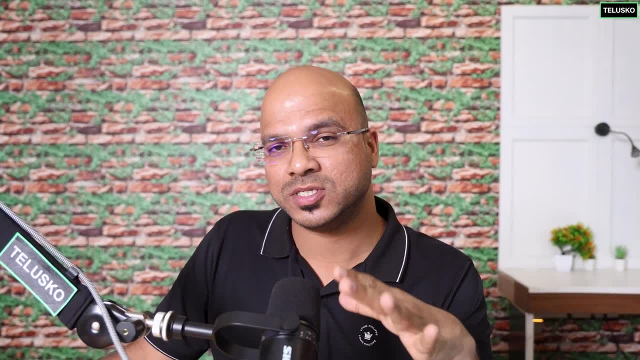 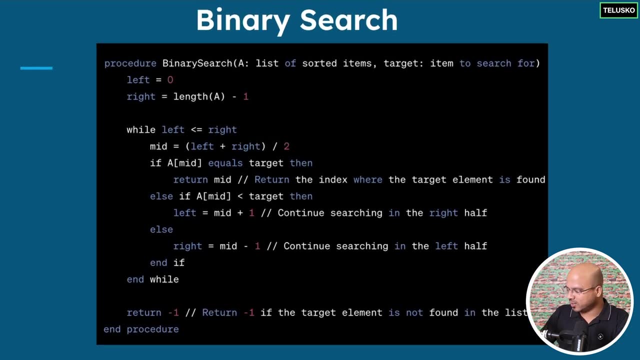 right, It will take a lot of time for binary search, But in general binary search works faster. But how do you do that? So, with this theory, let's talk about the practical implementation of binary search. So let's look at the code here very fast, because we have already done the 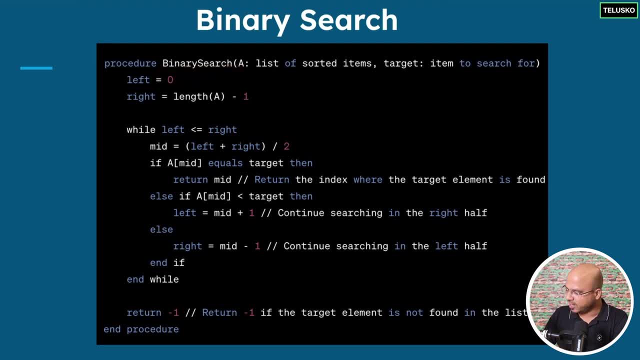 theory here. So what you do is you basically write a function, let's say binary search, and then you pass a list of values, right, And then you also pass a target- same thing we have done in the linear search- And here then you go with the left and right. So basically we have: 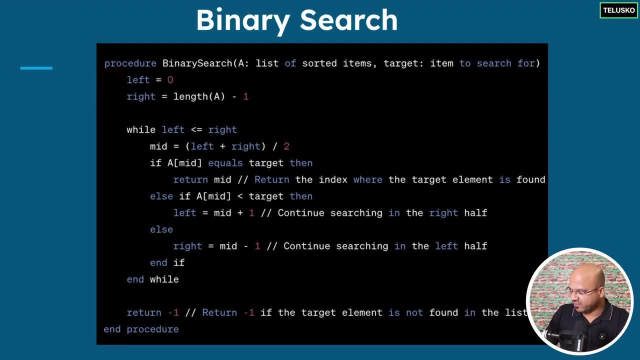 mentioned the start and the end Here. in this we are taking left and right. Left starts with zero, as we mentioned, the starting starts with zero, ending ends at the last value. Okay, we have done that. And then you run a loop till you find the value, of course. Then what you do is you check. 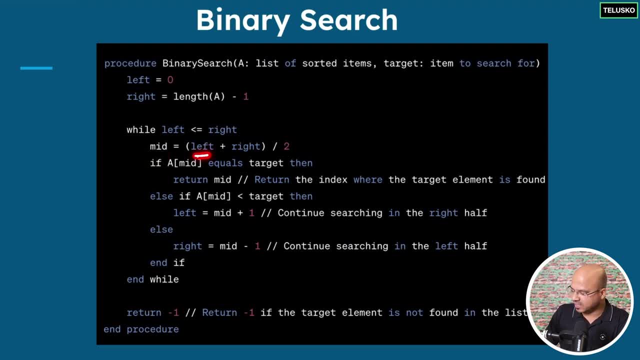 the mid value. So this is the mid value. we have done that. Mid is the starting point, ending point, divided by two, And then you check: is the mid matching with the target? If yes, you're done, you can simply return the value. Otherwise we have to do something more. Then you check. 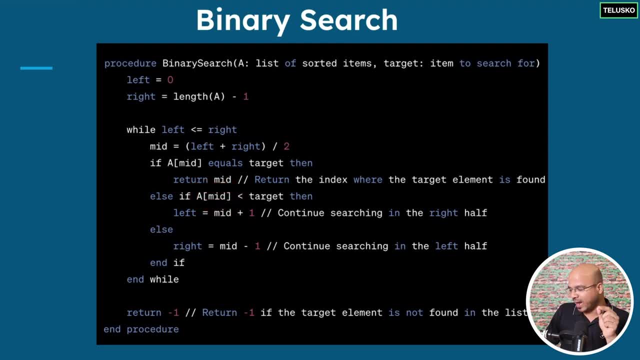 if the value which you got, which is mid value, and the target, if the mid value is less than the target, In this case, you will focus on the right hand side. Okay, so basically you have to shift to the right hand side. So your left, your starting point will shift And we have discussed that here. 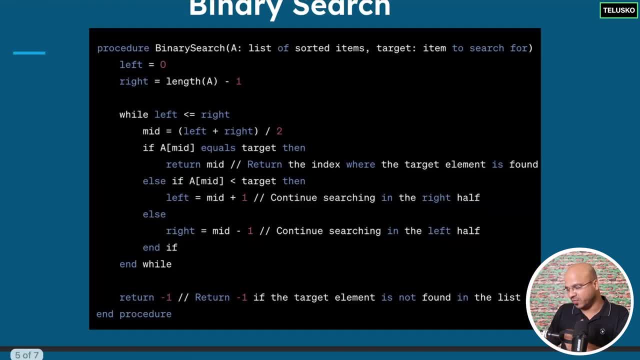 right, Your starting point will shift. And then what if the mid value is greater than the target value? In that case, you will shift to the left position. Okay, so that's what we have doing here. And then, every time you do that, you run the loop again, you find a new mid value, And that's what. 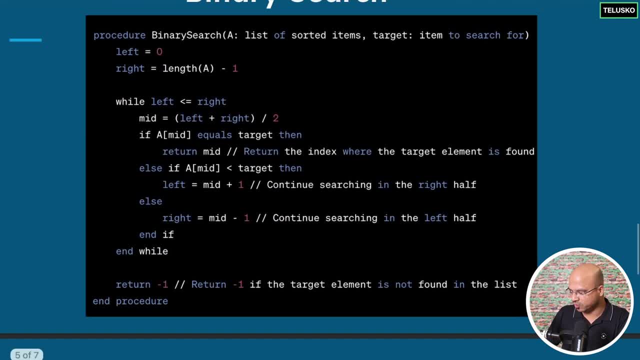 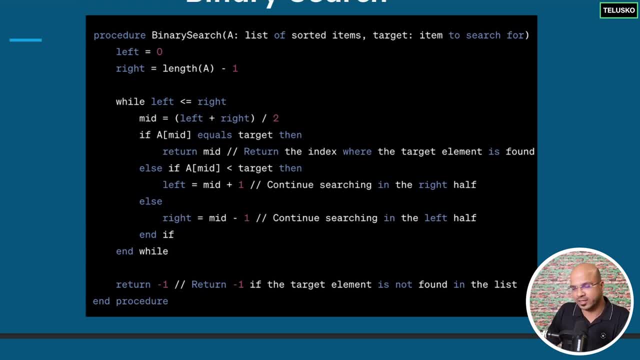 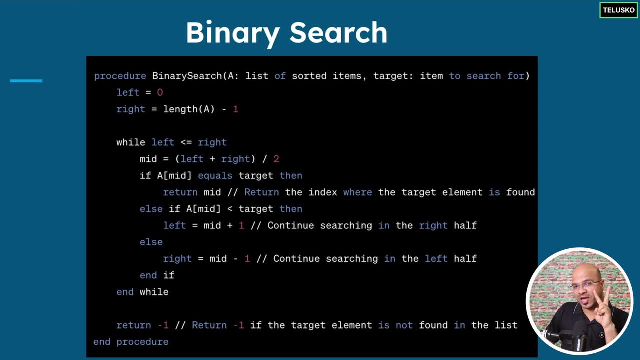 here And then, at the end, you will get a value. If it is not there, you will simply return minus one, as we have done before. So basically, by doing this, what we're doing is we have seen two algorithms. right Now we have to find the time complexity. Now, what exactly time complexity is? 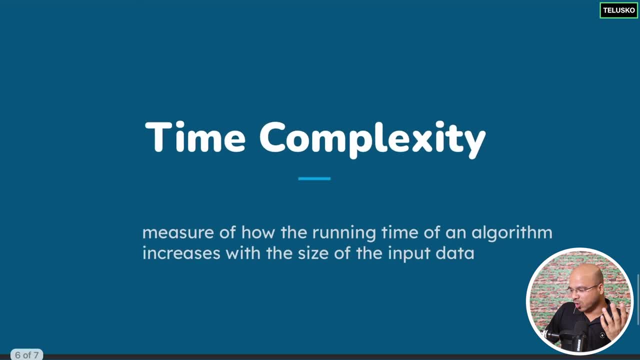 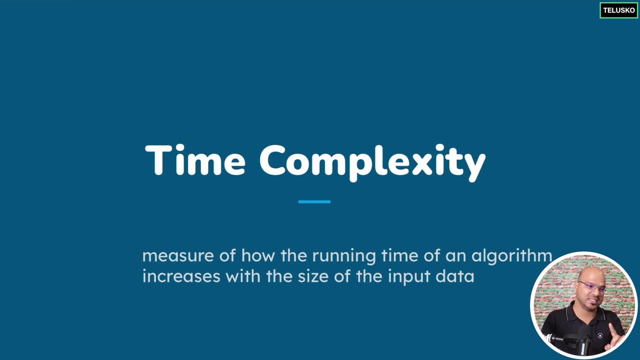 it's not about number of seconds it takes to run your code, It's all about this. So time complexity simply means the measure of how the running time of an algorithm increases with the size of input. So basically, let's say, when you are testing a particular algorithm you're testing for. let's say, 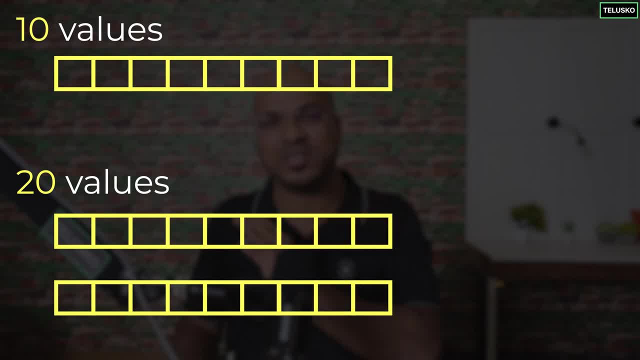 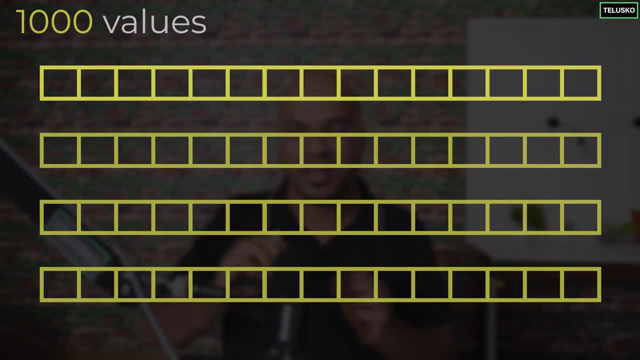 10 values or 20 values. But what if the values goes up? What if you have 1000 values? How will it will affect your time? Will it increase the time in linear section? Let's say, if it takes five seconds for 10 values, will it take 10 seconds for 20 values, Or will it take more or 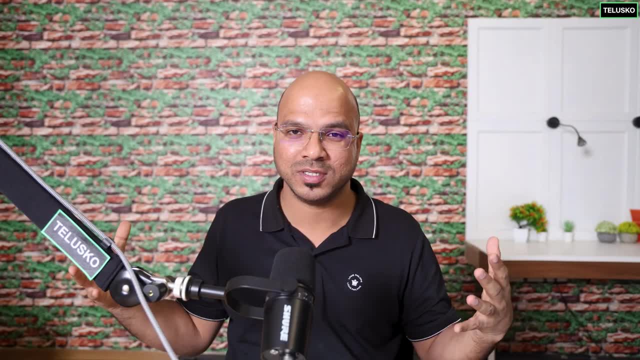 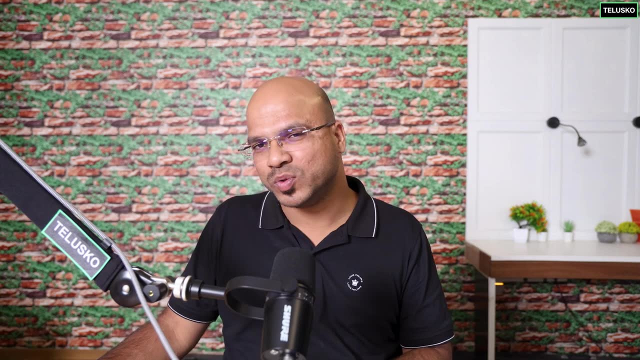 will it take less? Okay, or let's say, you have 1 million records, Will it take 1 million seconds? That's the question we have to answer. Okay, Now how will you do that? And that's where we have something called big O notation. Now what? 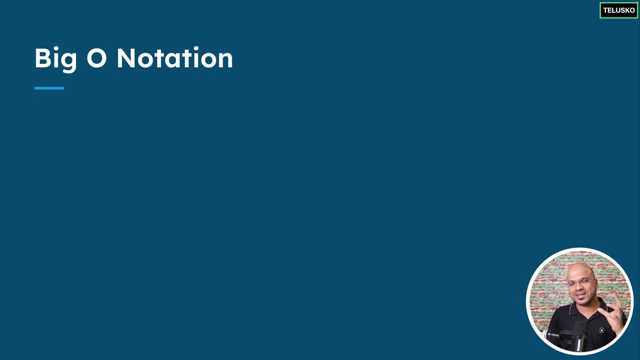 happens in big O notation is we use this particular concept to understand your time, complexity of your algorithm. If someone says, hey, your algorithm is not fast enough, you have to first find the big O notation of it. So why big O? is because it is represented with the help of O, the big O. 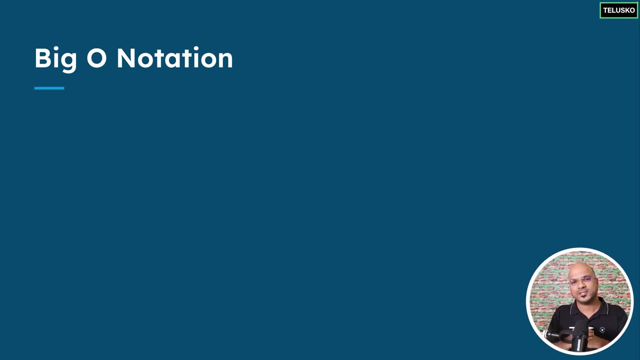 in bracket you mentioned the order of n or something. So basically it will also call the order of our big O notation and you anything will do. So how do you represent that? you represent that with something like this: So we have O of and then the value, which is one. 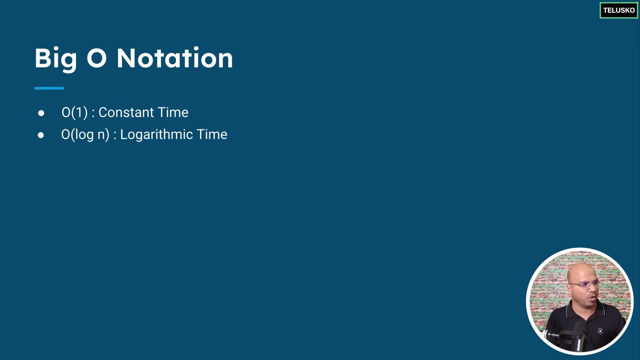 will keep changing, So there are multiple things here. you can say: we have O big O of log n, we got big O of n. we got big O of n log n. we say big O of n squared, which is quadratic time. 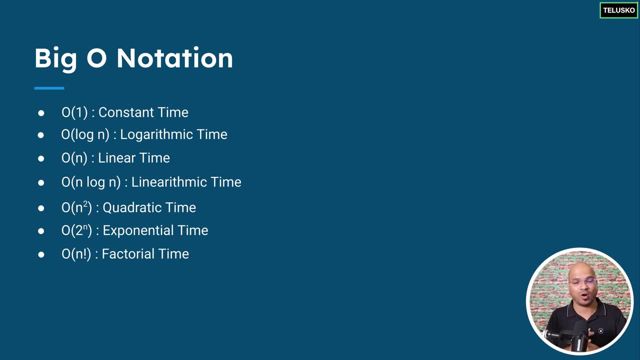 we got to this, to n, we got n- factorial, Okay. so we got all this notation, But how do you find this? Okay? now, this is tricky. So, of course, in this particular video is not, you will not understand everything, But let's start with the basic. Now let's talk about the linear search Now. 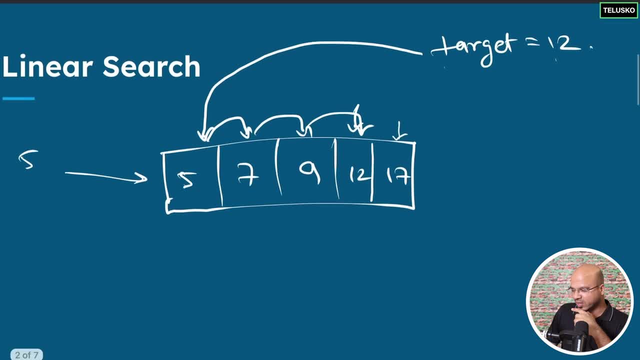 if you go back to linear search, what we were doing there Now, in linear search, when you have five values, you take five steps. when you have 10 values, you take 10 steps. you. when you have 100 values, you take 100 steps. right. But let's say that is for searching, right? What about? 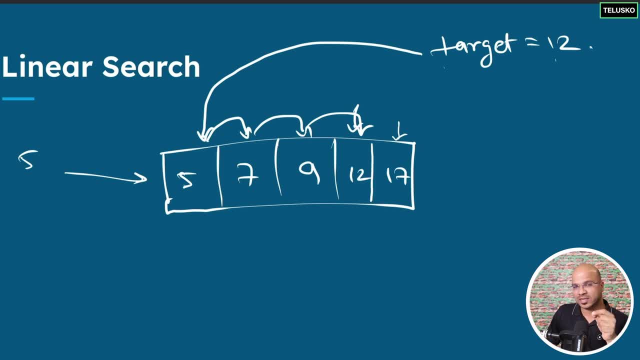 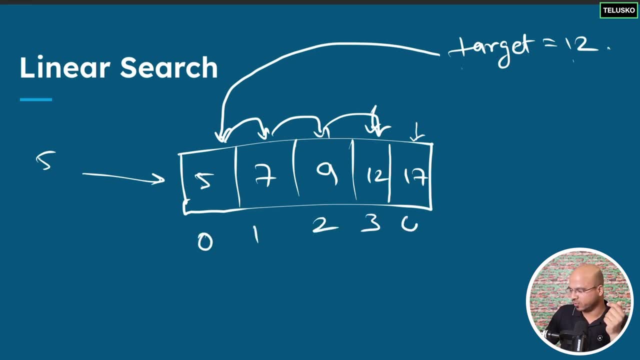 reading. If you want to read a particular element from the linear search or from the array, it's very easy, right? You specify the index value. let's say the index value is 01234.. And then you specify: hey, I want the value at index two. So let's say you say nums, which is 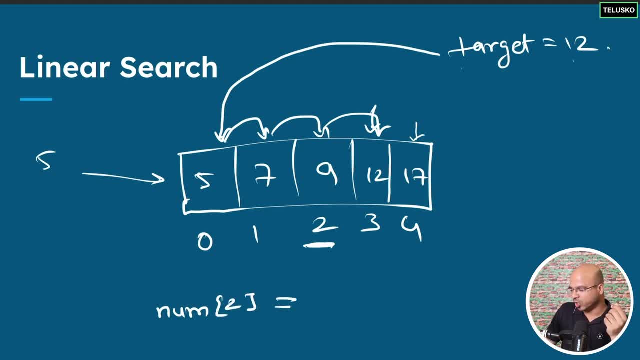 the name of the array, And when you say two, basically what you get is nine. it's very fast, So it doesn't matter what is the size of your array: it can be 1 million records. the time taken to get a particular element with the help of index value is constant, right, Because computer knows. 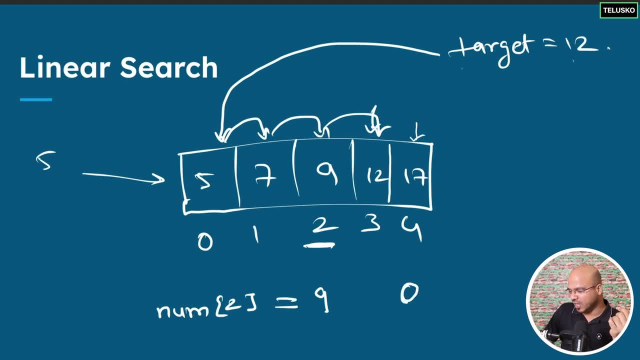 what memory is. So in that case I can say the big O, the time complexity for this is one, because it is constant. Okay, now see, it's not about one step. if you're thinking, just because I mentioned that it is only one step, it can be three steps as well. So let's say, if you are reading a particular 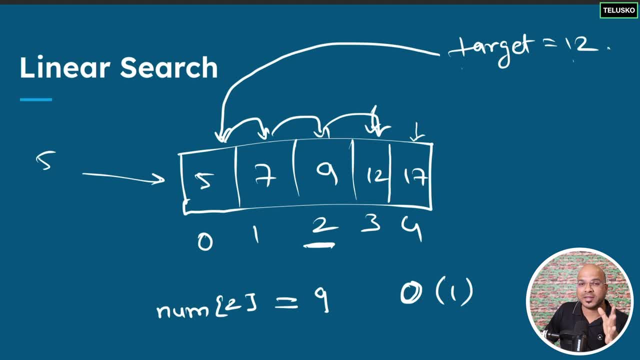 element and maybe behind the scene it takes three steps. doesn't matter, It's constant, right, It can be one step, three step, 10 steps. it should be constant. If it is constant, you can say O of 1,. 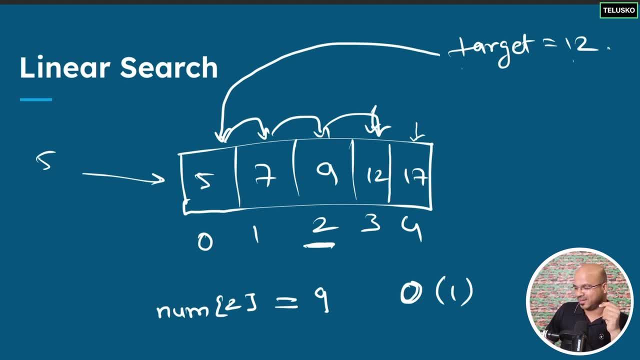 but what if you are searching element? So if you have an array size of, let's say, 10, it takes 10 steps. Now you'll be saying, hey, you know what? if the element is at the start itself, of course it will take one step. But we have to go for the worst case scenario here, The worst. 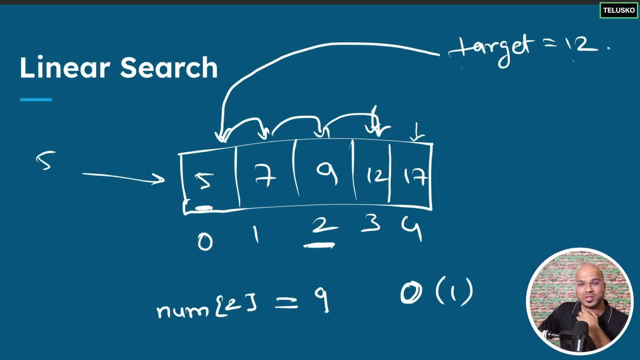 case is, what if the element is at the end? What if the element is not even there? it will take 10 steps And that's why we can say the order. the big O notation here will be n. what is n here? the? 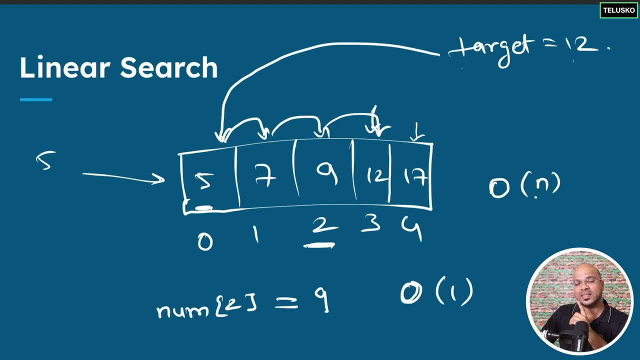 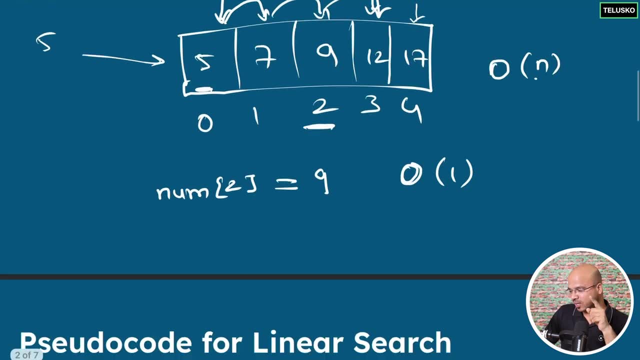 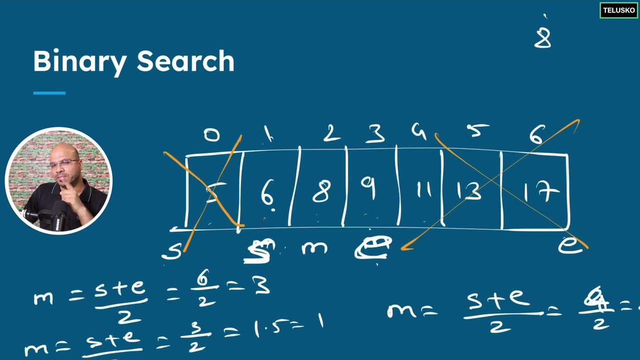 number of elements in the array. as it increases the time also increases the time complexity. I'm not talking about the actual seconds. Okay, so that's your linear search. Now, coming back to the binary search, what could be the big O notation for binary search? See, the thing is as the number 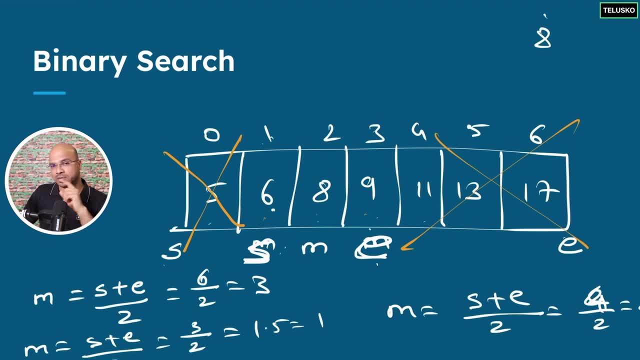 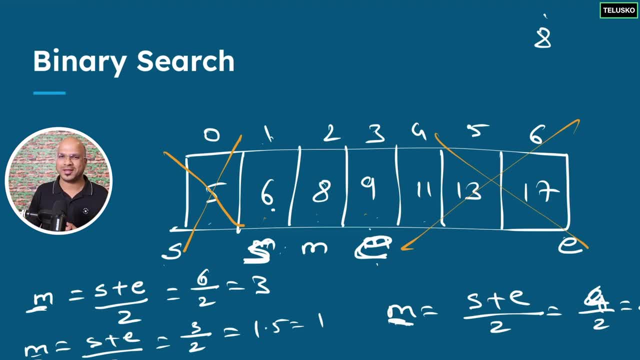 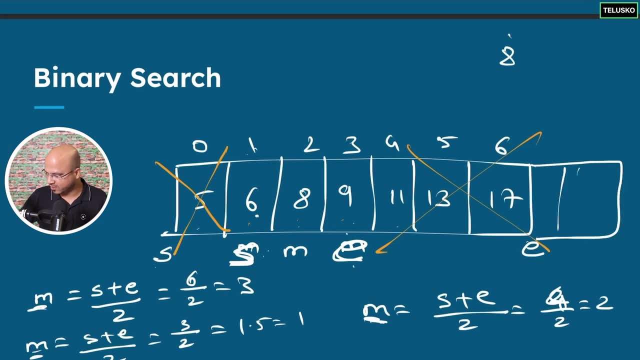 to double. So let's say, from seven we got 14.. So what do you think? how many steps will increase? What if I say, only one reason being even if you have, let's say, 14 values here, let's say we have. 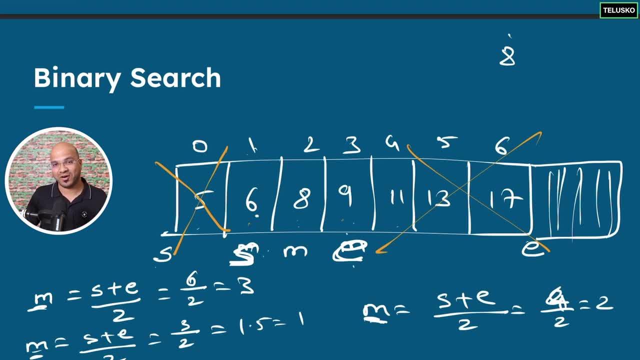 so many values at the start itself it will be half right. you will get seven values after one step And then you basically include, increase one more step to find the middle. So that means when your value increases it will also increase the number of steps taken, but not exactly n Because 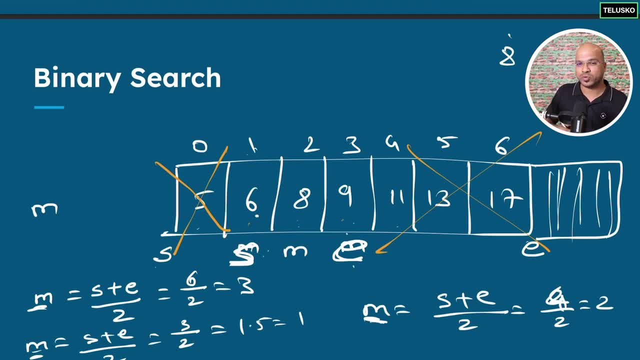 in the linear search. if your number of steps increases, it will also increase the number of values increases by 10, it will increase 10 steps Here. as the number of value increases, it will not increase the steps in the same sequence. So what we can say is: we can say it is something. 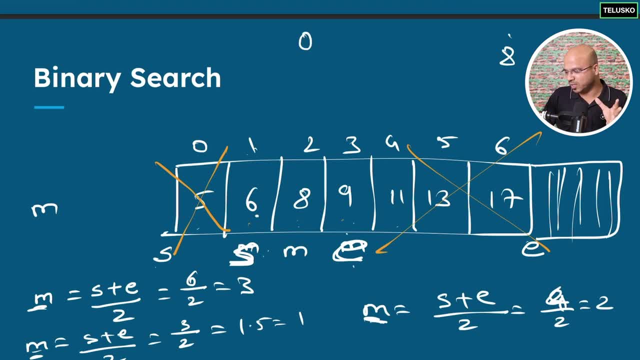 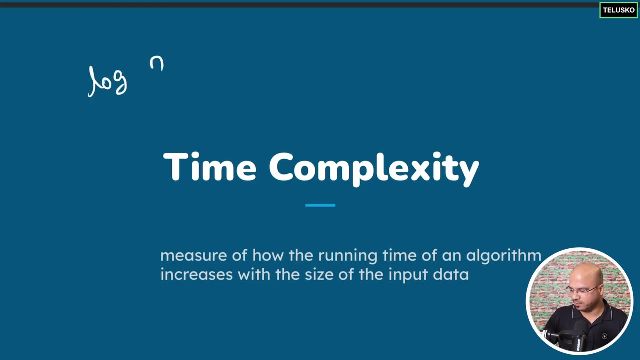 between constant is not exactly constant, but it is between the O of one and O of n. So it is between this two, And what comes between this two is O of log n. Now, what is log n basically? so log n basically means we have a base two here by default, okay, so number of steps it takes. So what exactly this? 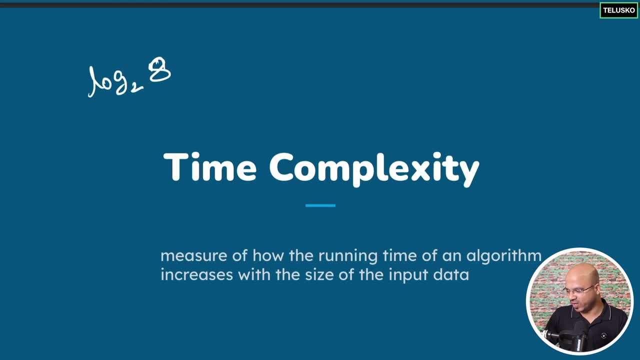 n here. so let's say we have eight values here. So when you say log two of eight, it will give the value which is three. Okay now, why it is three is because log of eight is simply means it will take to multiply itself three times to get eight. Okay, so as the number increases, 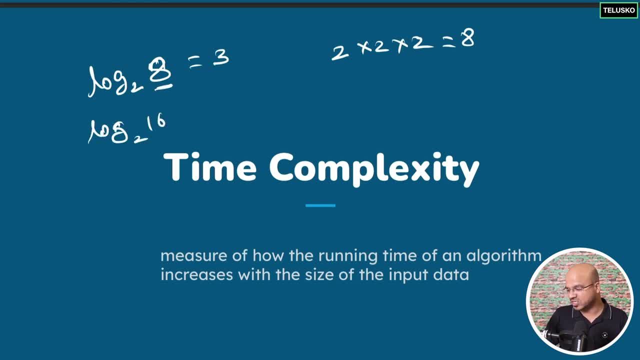 let's say now, instead of eight values, we got 16 values. it will give you four, because it will take two to multiply itself four times to get 16.. Right, So it will give you four. that means, as your number of value increases from eight to 16, it will only increase one step right, And that's. 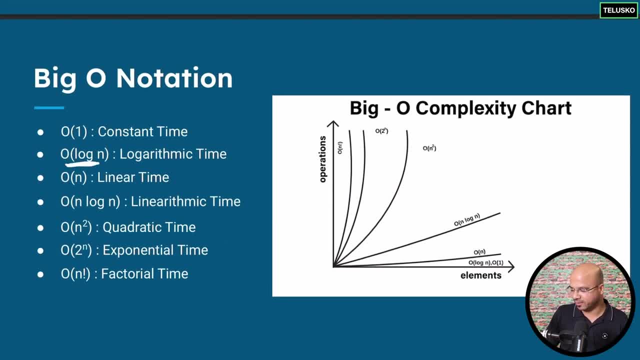 why the binary search is log n. So your linear search is O of n and your binary search is O of log n, So, which will take less time, the log of n. Okay, And you can see the graph here as well. So, 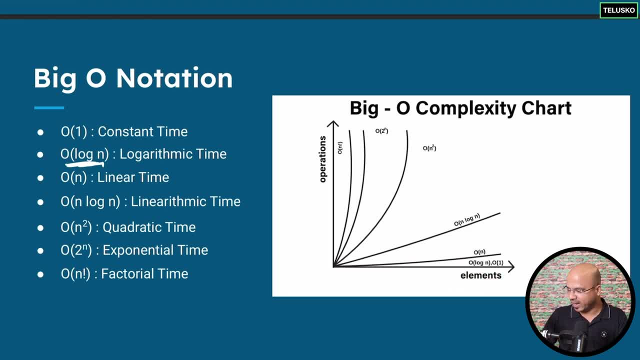 this is elements, the number of elements you have in the array, And this is the number of operation it takes. Okay, so number of steps. So if your algorithm is following the constant time, it means it's here. it doesn't matter how many values you increase, it will be constant time. log n is similar to it's almost. 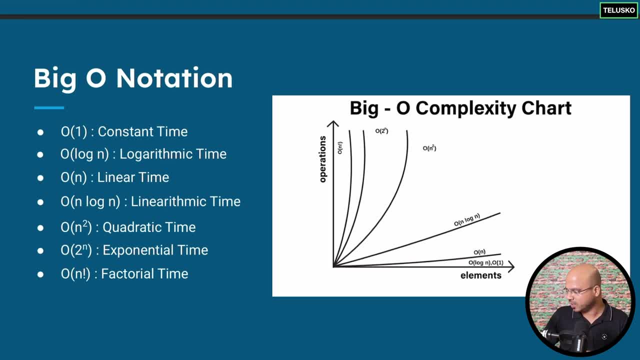 same as constant. not exactly same as constant, but it will take less time. So you can see. log n is mentioned here. It's there. the wave is there. you can't see it, it's there. So what if you go? 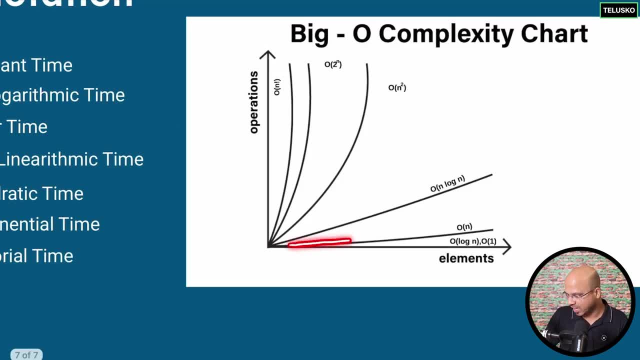 with big wave, O of n. so as your value increases, your time also increases, right. But there can be some worse scenarios as well. there can be some other algorithms which you implement which might take n log of n which is worse than O of n. there might be some algorithm which will take O of n. 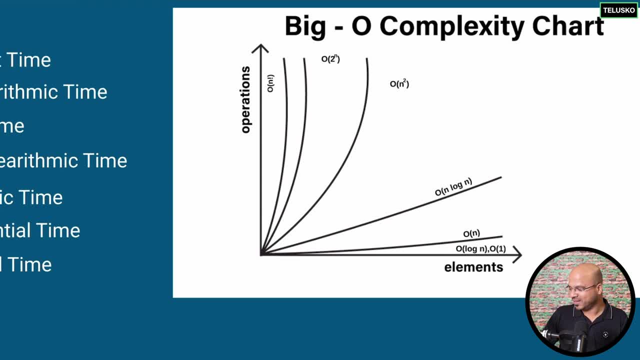 squared, which is worse than the O n log n. So, basically, if you want to build an algorithm, try to make sure that you are here. if you are here, you're good. Okay, if you are here, it's better. However, if you are here, try to make it better. If you are here, that's the worst scenario. 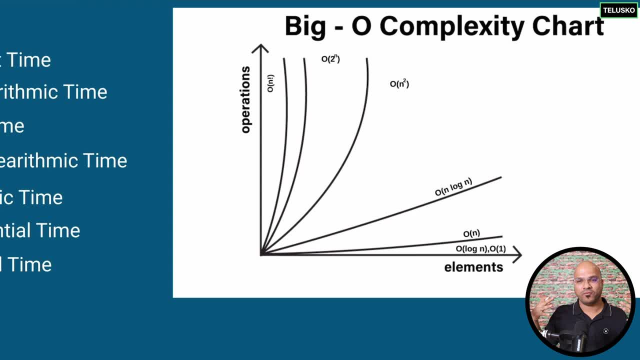 that means you're building an application which is not scalable. The moment you have five users on your server, your server says: I'm good. The moment you have 1000 users, it will struggle. Okay, so make sure that which of the algorithm you write, you follow this. 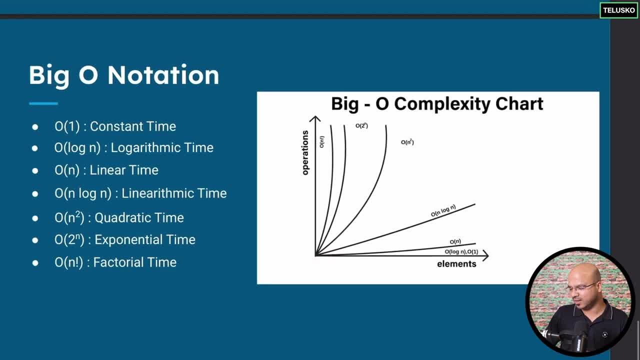 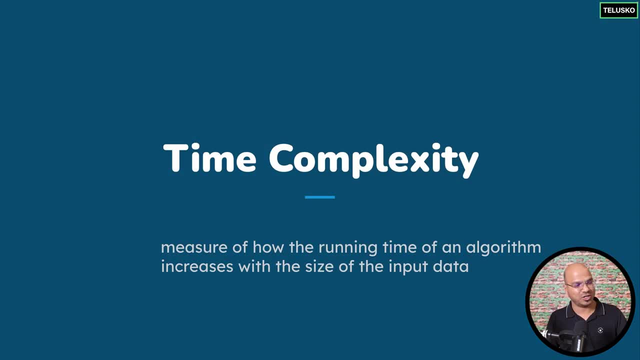 Of course, in the upcoming videos we'll work on some more algorithms. we'll see which one matches there, But you've got the idea right. So the time complexity set simply means this definition: the measure of how the runtime of the algorithm increases with the